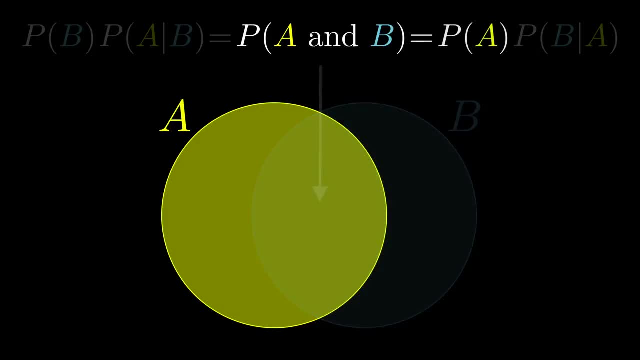 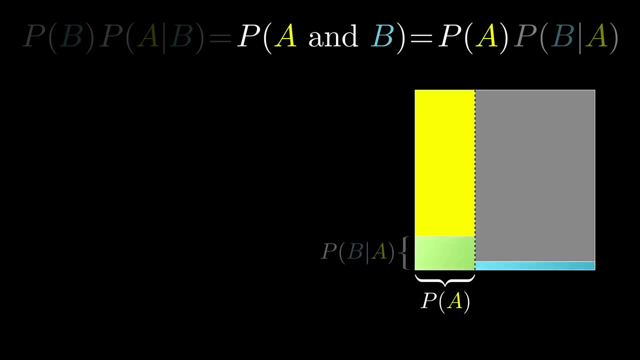 of them happen. On the one hand, you could start by thinking of the probability of A, the proportion of all possibilities where A is true. then multiply it by the proportion of those events where B is also true, which is known as the probability of B given A. But it's strange. 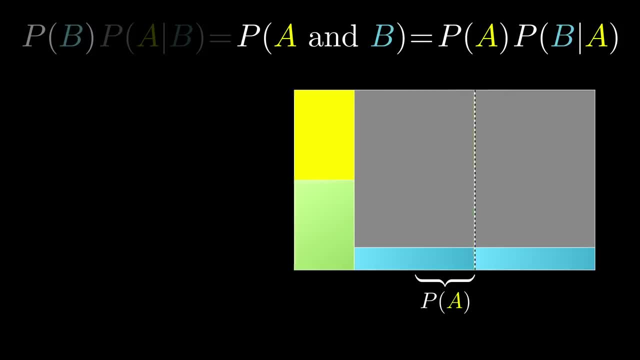 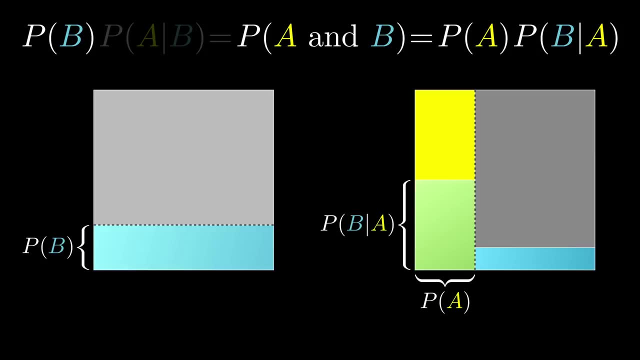 for the formula to look asymmetric in A and B, Presumably, we should also be able to think of it as the proportion of cases where B is true among all possibilities times the proportion of those where A is also true, the probability of A given B. These are both the same. 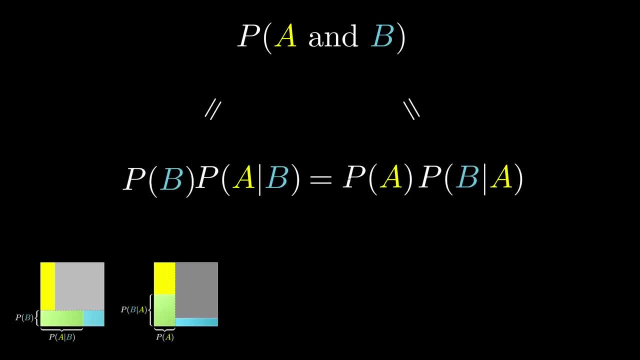 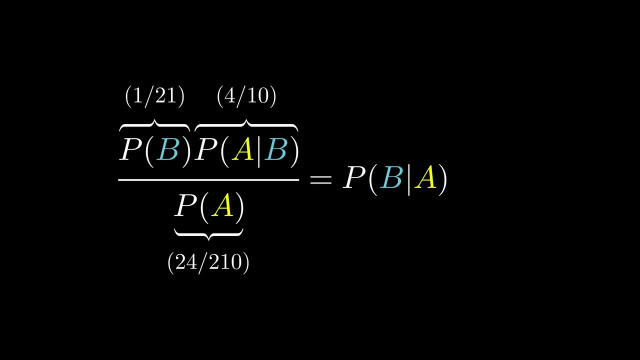 and the fact that they're both the same gives us a way to express P given B in terms of P. So when one of these conditions is easier to put numbers to than the other, say when it's easier to think about the probability of seeing some evidence given, 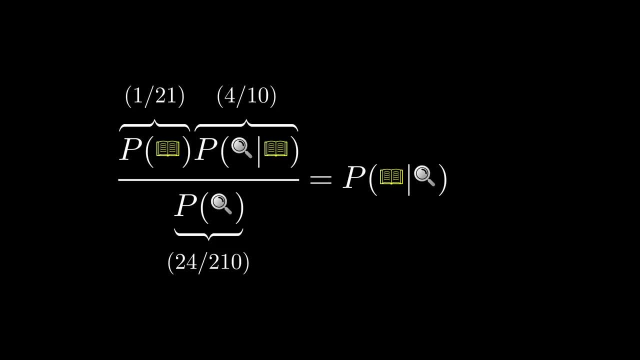 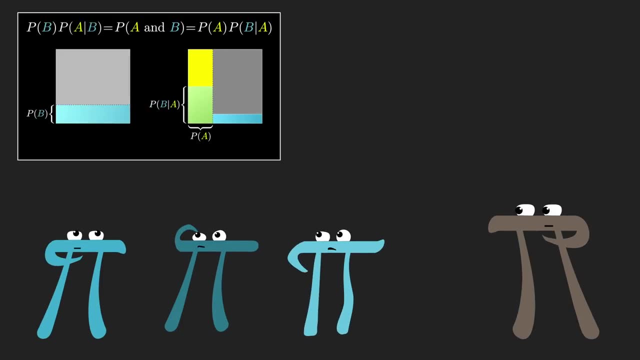 a hypothesis, rather than the other way around. this simple identity becomes a useful tool. Nevertheless, even if this is somehow a more pure or quick way to understand the formula, the reason I chose to frame everything in terms of updating beliefs with evidence in the main video. 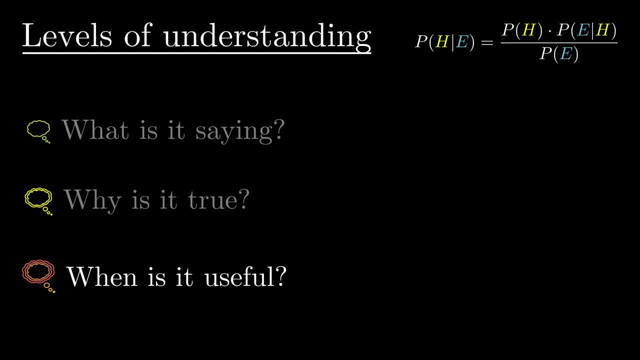 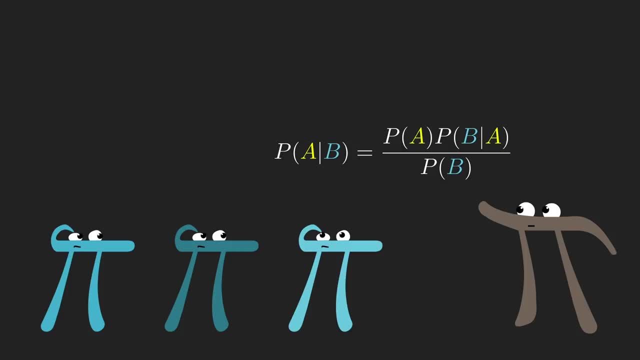 is to help with that third level of understanding: being able to recognize when this formula, among the wide landscape of available tools in math, happens to be the right one to use. Otherwise, it's kind of easy to just look at it, nod along and promptly forget. 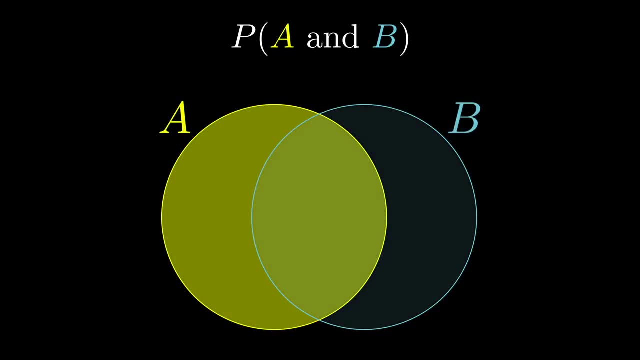 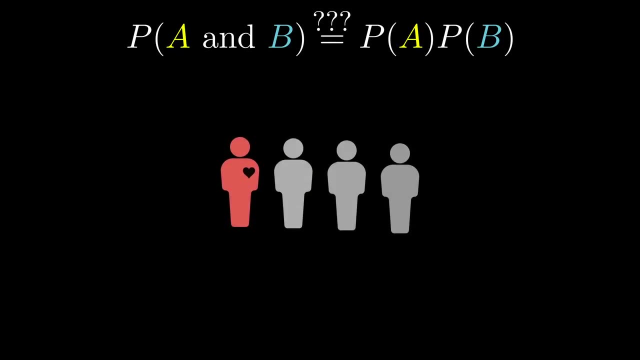 And you know, while we're here, it's worth highlighting a common misconception: that the probability of A and B is P times P. For example, if you hear that one in four people die of heart disease, it's really tempting to think that that means the 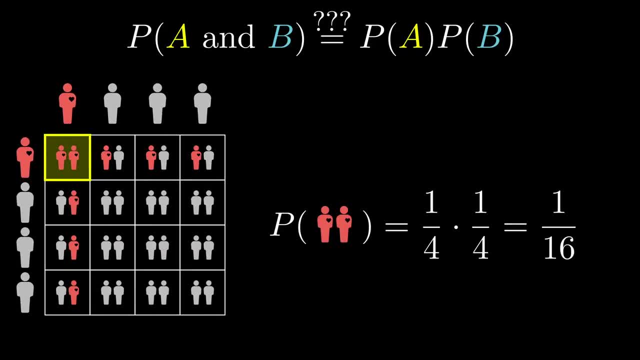 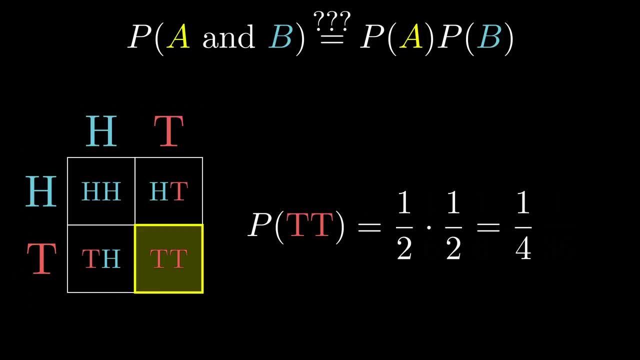 probability that both you and your brother die of heart disease is one in four times one in four, or one in sixteen. After all, the probability of two successive coin flips yielding tails is one-half times one-half, and the probability of rolling two ones on a pair of dice is one-sixth. 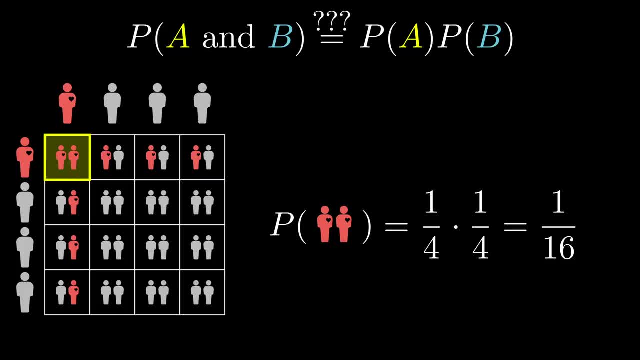 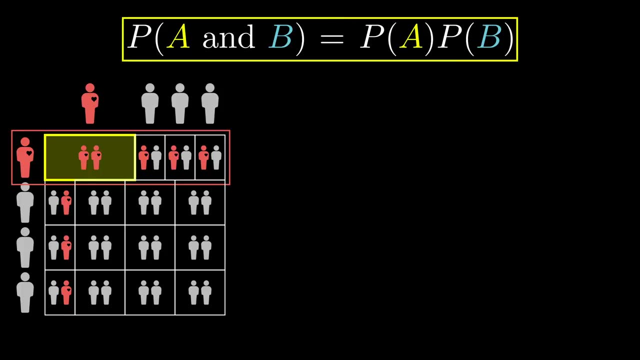 times. one-sixth right. The issue is correlation. If your brother dies of heart disease, and considering certain genetic and lifestyle links that are at play here, your chances of dying from a similar condition are higher. A formula like this, as tempting and clean as it looks.